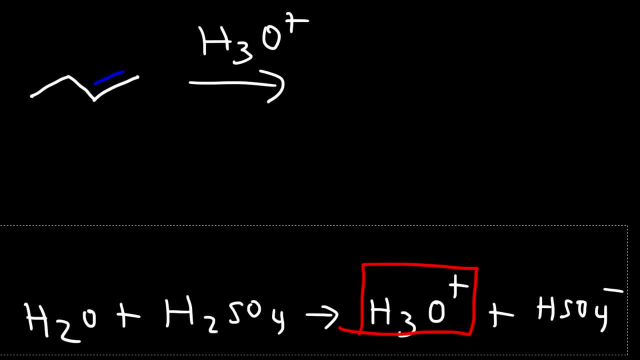 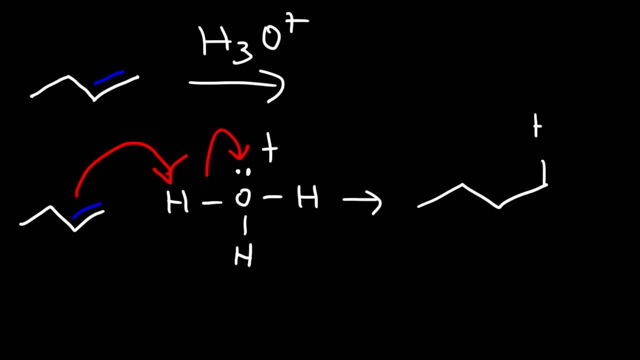 would produce the same result. So what's going to happen here? The alkene will react with H3O plus. The double bond is going to attack the hydrogen atom much the same way as it reacts with HBr, and then the OH bond will break. Now the hydrogen atom will go on the less substituted carbon atom. That 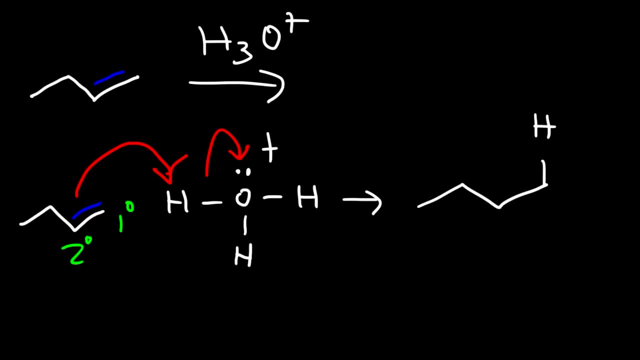 is the primary carbon atom of the double bond, so that we can get a more stable secondary carbocation. Now, once we take off a hydrogen from H3O plus, it becomes water. So in the next step, water is going to add itself to the 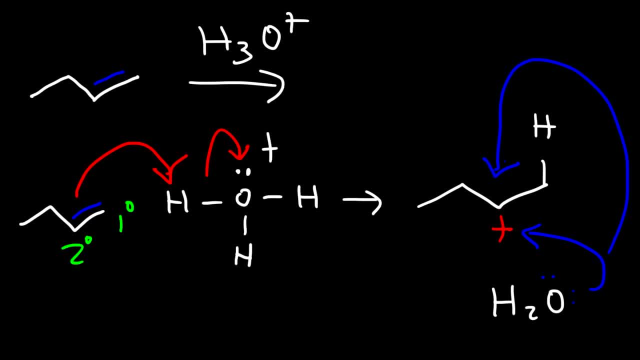 carbocation. It can attack from the front or it can attack from the back, So we can get a racemic mixture of products. But first we're going to get the oxonium ion species, which looks like this: Whenever oxygen has three bonds, it 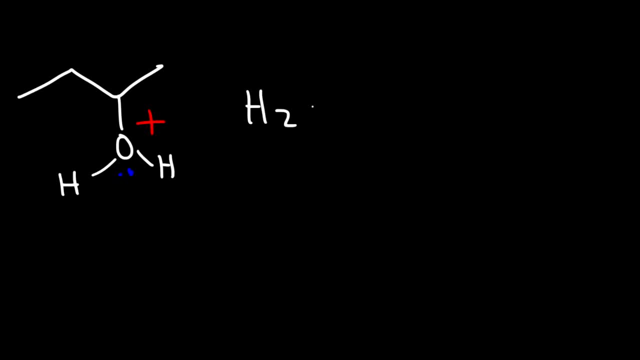 has a positive charge, And then we need to use another water molecule to remove this hydrogen, And so now we have our final product, which is an alcohol. Now, this is a chiral carbon. So really, we have two different stereoisomers. We have both R and S, two butanol, So these are the products for this reaction. 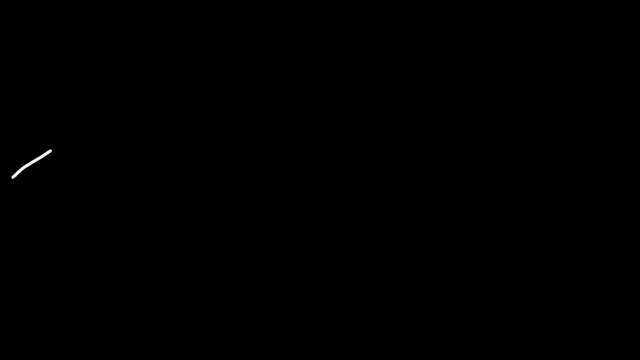 Now it's important to understand that the acid catalyzed hydration of alkanes is in equilibrium, So this reaction is reversible. It's based on the concentration of the acid and also the temperature. So, for instance, let's say, if we add water to an alkene, Neutral water won't react with this. 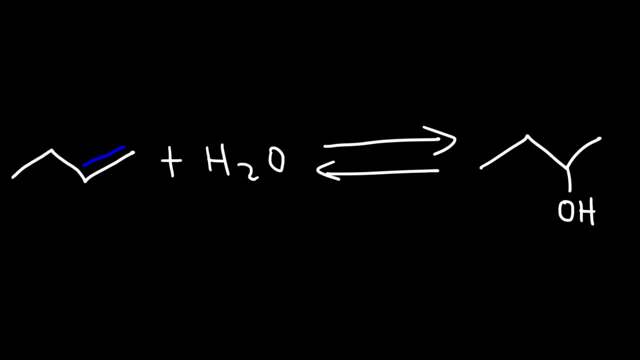 alkene at a very significant rate. But if we add dilute acid, it will catalyze the reaction, speeding it up. Now, if we add concentrated sulfuric acid, the reaction will go towards the left. Concentrated sulfuric acid reacting with an alcohol. 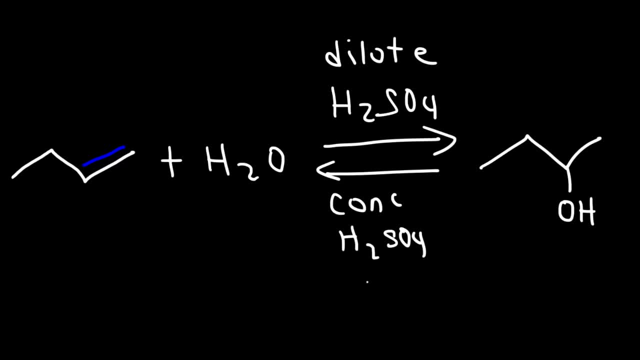 can give you this alkene by means of an E1 dehydration reaction. And so, if you think of Le Chatelier's principle, if you increase a reactant, the reaction will shift to the right. So let's say, if you increase the 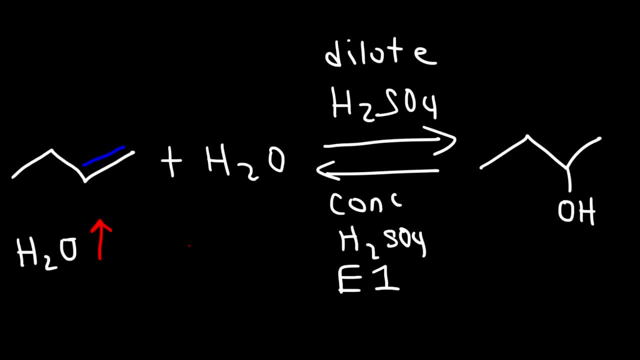 concentration of water, then the reaction will shift to the right, to produce more product, more alcohol, And so you can have a greater concentration of water when you have a dilute sulfuric acid solution. Now, if you decrease the concentration of water, the reaction will shift to the left, And that will happen if you have a 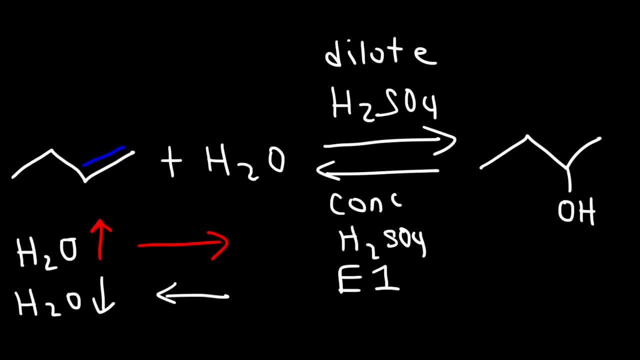 concentrated sulfuric acid solution, It's going to go towards the left to produce the alkene. Now, temperature is another factor. High temperature favors E1 dehydration And low temperature favors addition reactions. So if you want to make the alcohol, you want to use dilute sulfuric acid at low temperature. If you 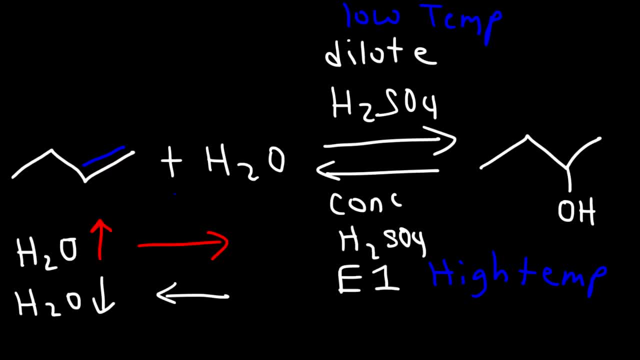 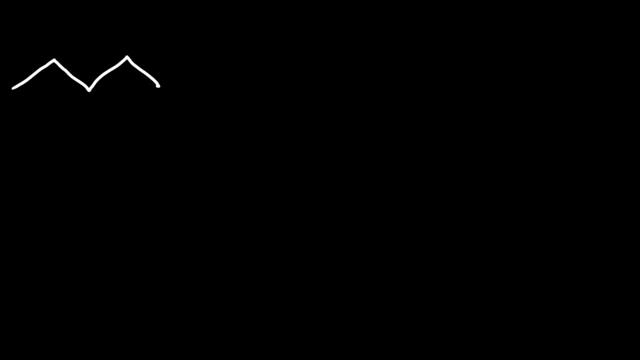 want to convert the alcohol back to an alkene, you need to use concentrated sulfuric acid at a high temperature. Consider this reaction between 1-pentene and methanol. We're going to react this alcohol with methanol under acidic conditions. So we saw what 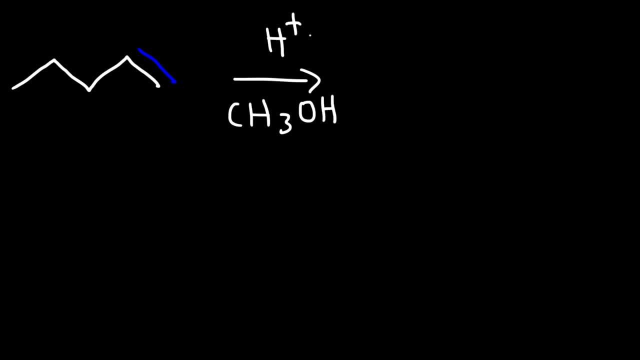 happened if we added water to an alkene under acidic conditions? But what if we add an alcohol to an alkene? What do you think is going to happen? Well, the first thing that's going to happen is the double bond is going to react with an acidic hydrogen, And so 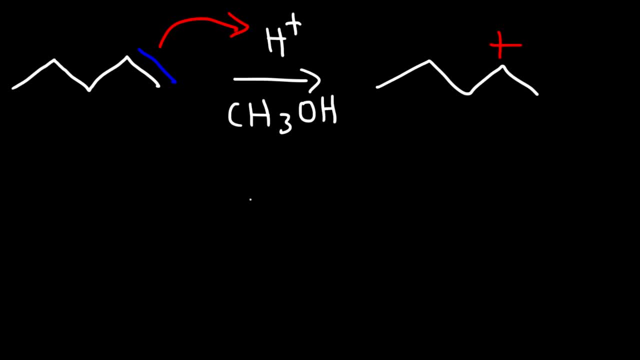 we're going to get a carbocation. We're going to add the hydrogen to the primary carbon, So this gives us a more stable secondary carbocation. And then the methanol molecule. it can attack the carbocation from either side, Giving us a racemic mixture. But first we're going to get this product, So this 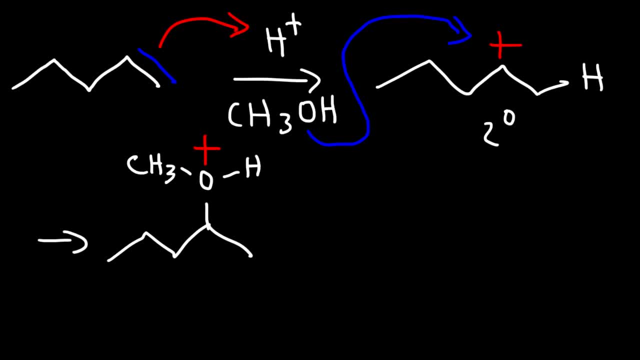 oxygen will have a positive charge And it will have one lone pair. And then we need to use another methanol molecule to remove the hydrogen, And so our product is an ether, But we're going to get a racemic mixture. So whenever you add an alcohol to an 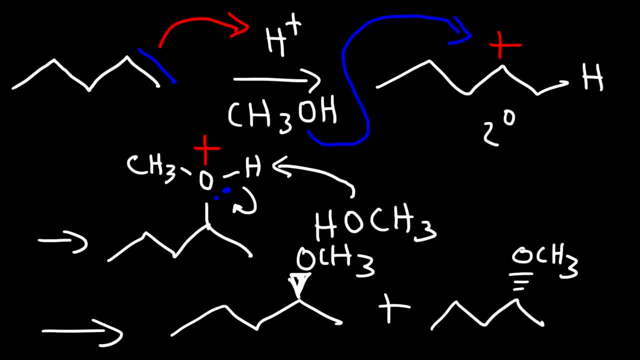 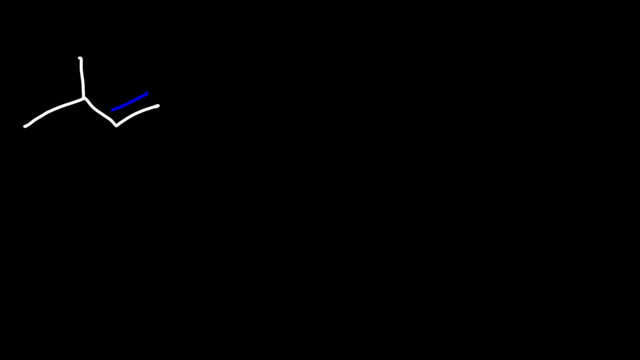 alkene under acidic conditions, you're going to get an ether. Let's work on another example. So let's react to this alkene with H3O+. Feel free to pause the video and try this problem. Go ahead and predict the major product of this reaction. So the alkene will react. 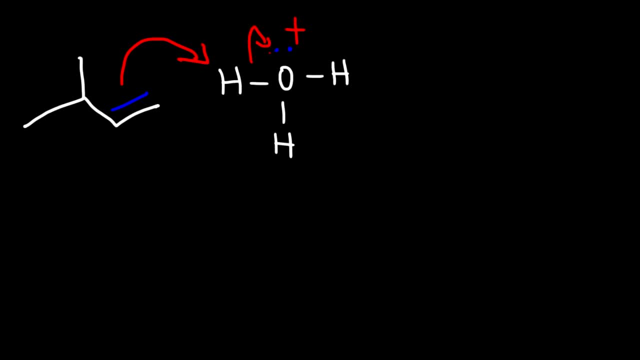 with the acid. It's going to take a hydrogen atom And the hydrogen, as always, will go on the less substituted carbon of the double bond. So it's going to go on a primary carbon, allowing the plus charge to be on the secondary carbon. Now 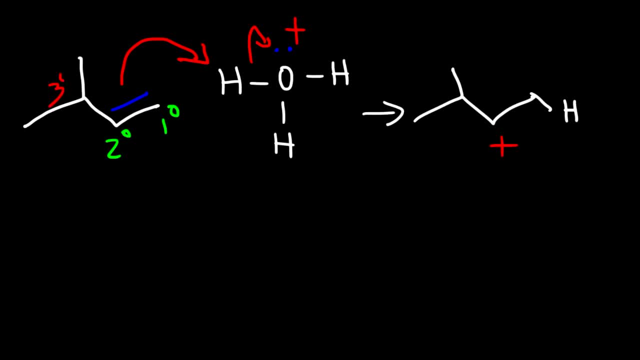 this plus charge is adjacent to a tertiary carbon, And so whenever you see that a hydride shift will occur, So this hydrogen will basically glide towards this positive charge. And the driving force is stability, Because a tertiary carbocation is more stable than a secondary carbocation, And so that's. 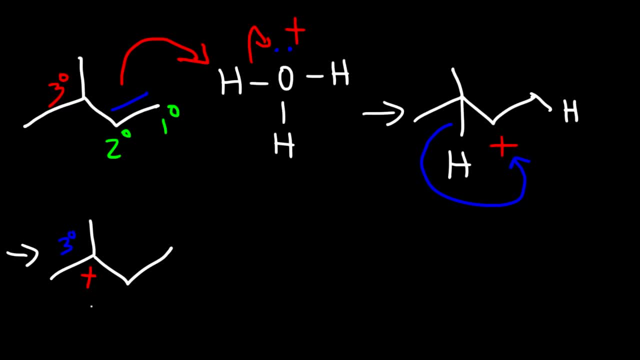 why this is going to happen. Now, once we have the tertiary carbocation, we can now react with H2O, So we're going to get this species, And then, for the last step, we need to use another water molecule to take off. 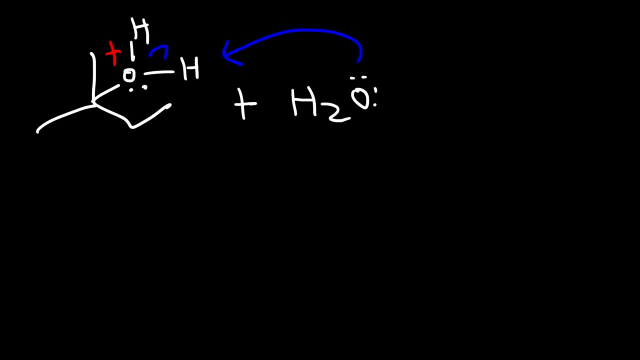 the hydrogen. And so now we have our final answer. This carbon is not chiral because we have two methyl groups attached to it, So we don't get a racemic mixture of products in this example. So this is the answer. Here's another reaction for you. 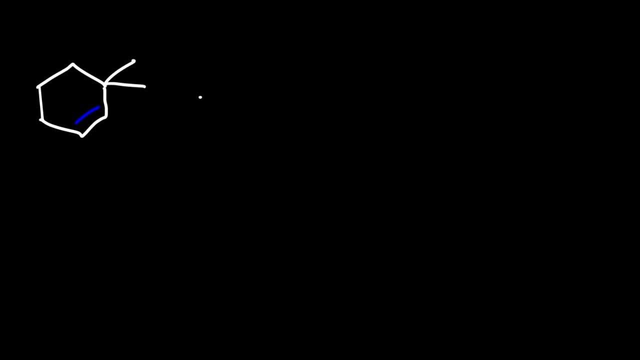 Go ahead and predict the major product with this reaction. So let's use H plus and methanol once again. So, as always, the double bond will attack the hydrogen. The electrons will flow from the nucleophile- in this case the double bond- to the electrophile, which is H plus. So, 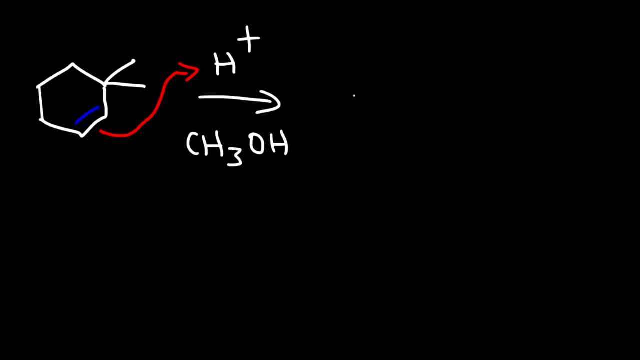 these reactions are known as electrophilic addition reactions. Now both carbon atoms are secondary, And so we can get a mixture of products. But here's the question for you: Is it better to put the hydrogen on this carbon And put the plus charge here, Or is it better to put the hydrogen on the other? 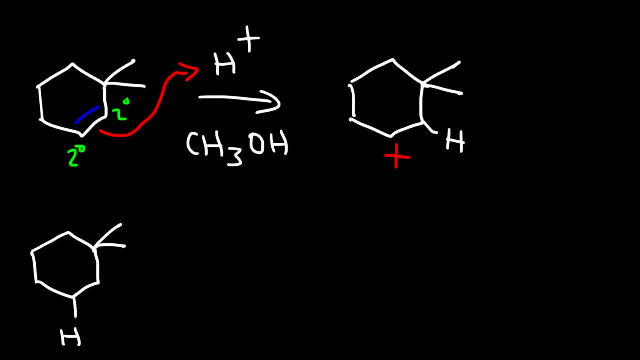 carbon of the double bond and have the plus charge in its location. As of now, both of these carbocations are relatively the same because they're both secondary carbocations. However, one of these carbocations has an advantage compared to the other one. 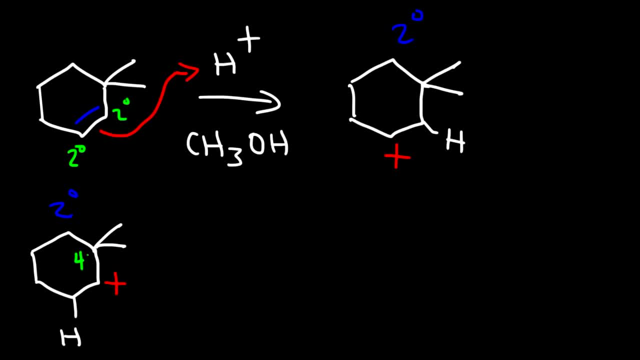 Notice that this carbocation is next to a quaternary carbon. As a result, it can become more stable by means of a methyl shift. So when the methyl migrates to this region, the plus charge is going to go where the methyl came from. So it's. 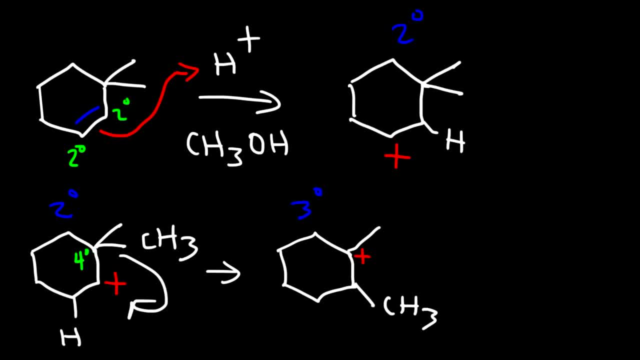 now in this carbon. So now we have a more stable tertiary carbocation. So now at this point the methanol will attack the carbocation And it can attack from the front or the back, And also when the methyl group migrated to this carbocation. now keep 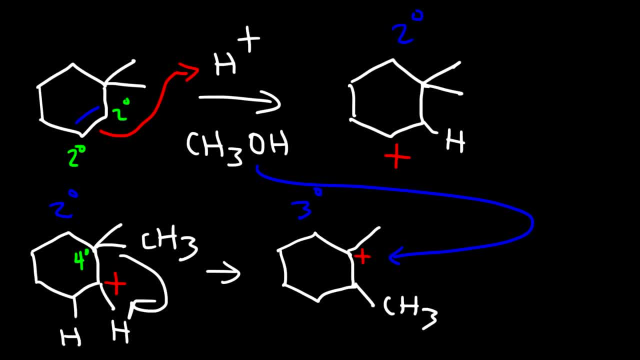 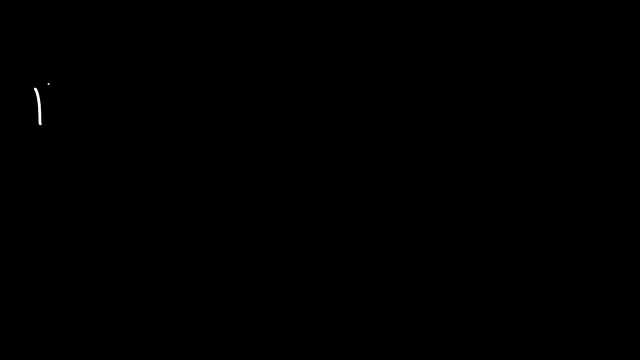 in mind. there's one hydrogen already present. the methyl group could be in the front or in the back, So we can get a mixture of stereoisomers in this problem, But for now this is what we have. So to complete the mechanism, we need one more methanol molecule to take off the 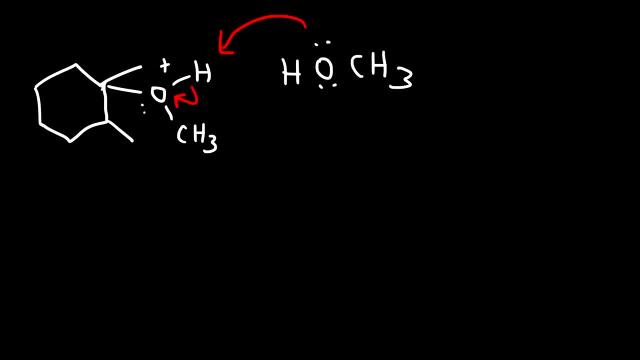 hydrogen, And so now we have our final answer, which is an ether. So because we had a plus charge at one point on both of these carbon atoms, and both carbon atoms are chiral, then we can get four possible stereoisomers. The methyl group can be in. 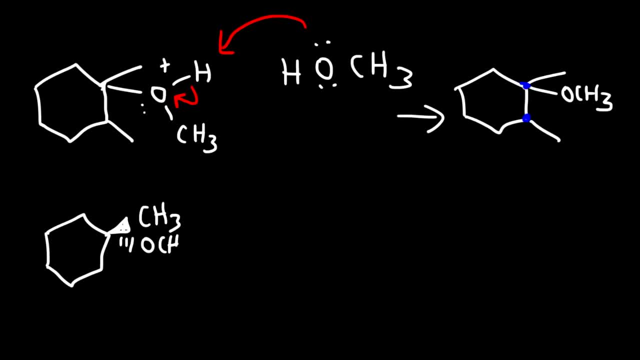 the front and the OCH3 can be in the back, And this methyl group can be in the back with the hydrogen in the front, And then you can get the other three stereoisomers. So you can get a mixture of four products. So if you want to draw, 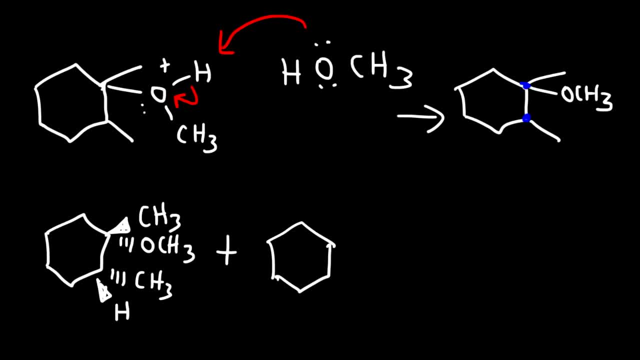 the next one. you could probably just change this chiral center, put in the methyl in the back and the OCH3 group in the front, And then you could change this chiral center if you want to. So you should get a. 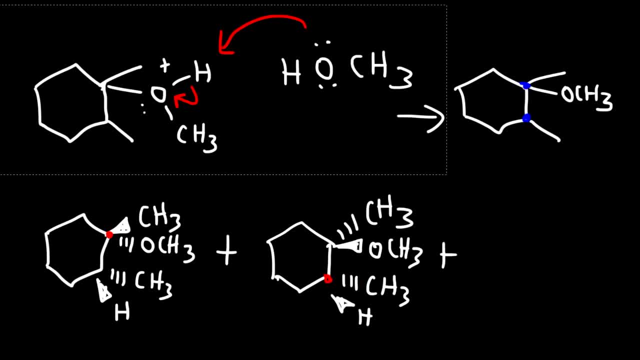 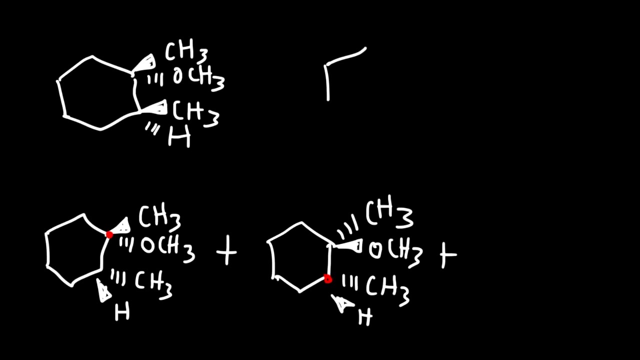 mixture of four products. So let me go ahead and draw the last two. So in this example, the CH3 at the bottom can be on the wedge and we can put the H on the dash. And for the last one, the methyl has to be on the dash at the top and the 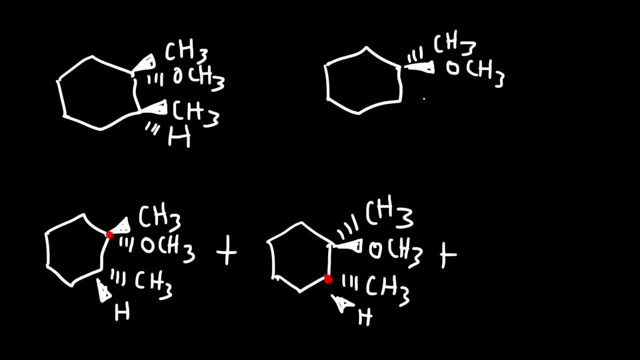 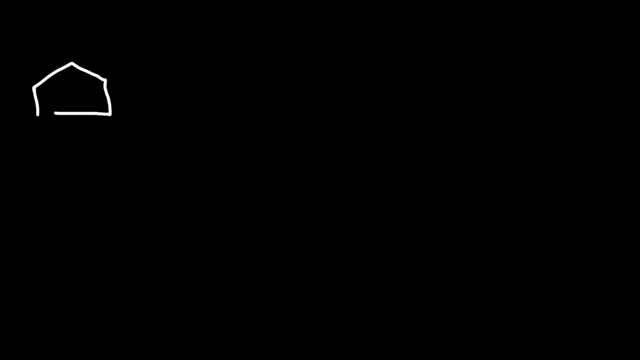 OCH3 has to be on the wedge, And then we're going to get this. So these are the four possible stereoisomers that we can get for this particular reaction. So here's the next example that we're going to go over. Let's react to this alkene with H3O+. 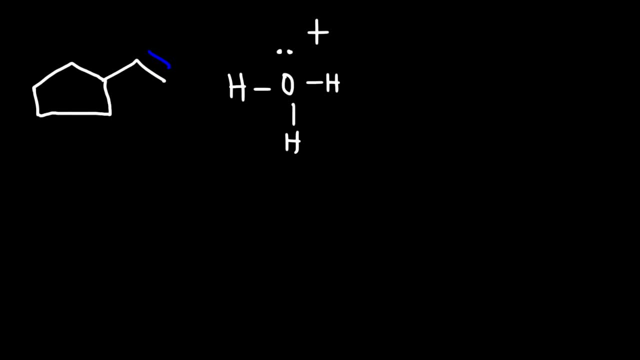 Go ahead and try it: Predict the major product for this reaction. So we know the first step: The double bond attacks the hydrogen and then the OH bond breaks Because oxygen is more electronegative than hydrogen. it's going to pull those. 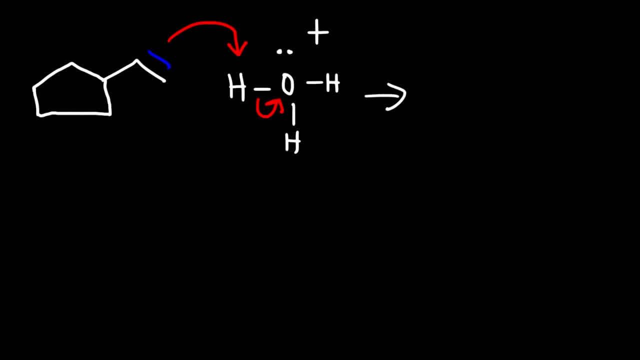 electrons toward itself And, as always, hydrogen will go on, the less-substituted carbon atom of the double bond, And so we're going to have a primary- I mean a secondary- carbocation. Now, what do you think is going to happen here If you have? 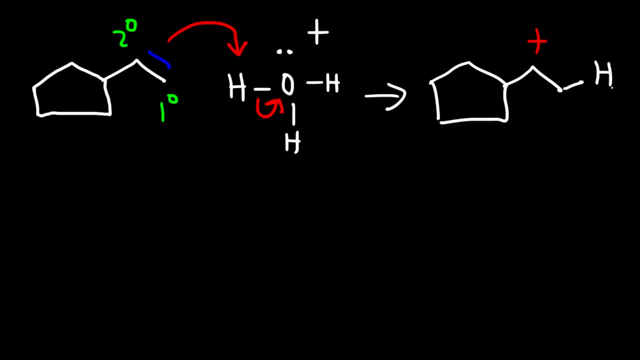 a five-carbon ring adjacent to a carbocation, typically you'll get a ring expansion, And so this bond is going to break. It could be this one too. It doesn't really matter which one you choose, And what's going to happen is as that bond. 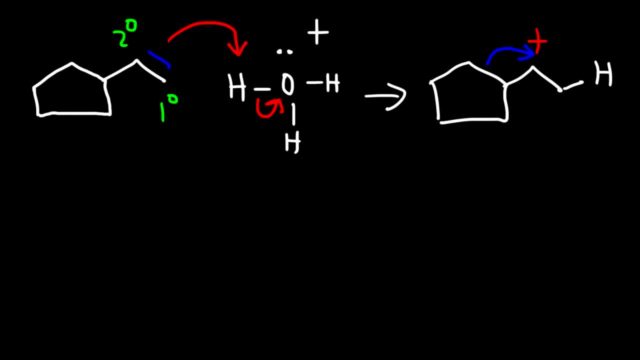 breaks. the electrons in that bond will be used to form the sigma bond between these two carbon atoms. So you're going to get a six-carbon ring. Let's call this carbon 1,, 2,, 3,, 4,, 5, and 6.. So let's draw a six-carbon ring And let's call this: 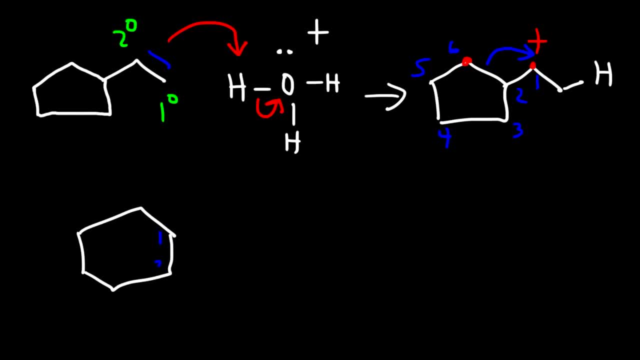 carbon 1.. And let's say this is 2, 3,, 4,, 5, 6.. Carbon 1 is attached to the methyl group And carbon 2 and 6 lost the bond, but a bond was formed between carbons 1 and 6. So because carbon 2 lost, 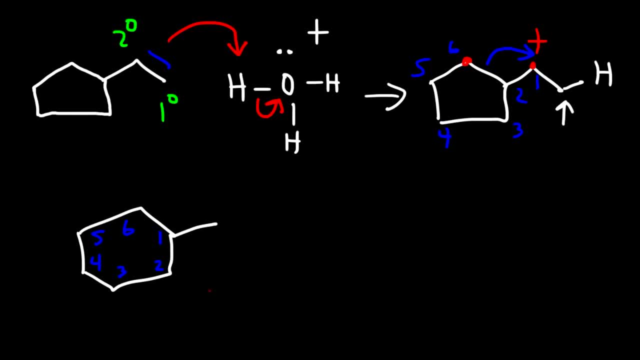 the bond and it didn't form a new bond. carbon 2 has the positive charge, So this is the structure that we now have. So what we have here is a secondary carbocation that's next to a tertiary carbon, And so whenever you see that a 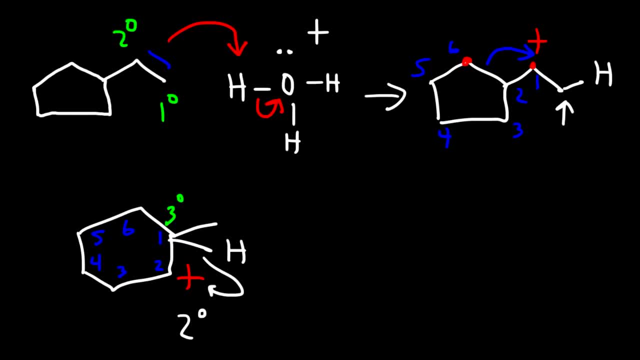 hydride shift will occur, So this hydrogen is going to move towards the carbocation, And so now what we have is a tertiary carbocation. So now let's talk about the rearrangements that just occurred here. So the first rearrangement was a ring expansion, And the reason for that is because the ring 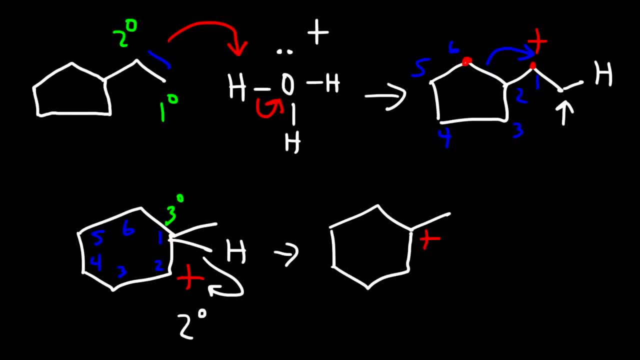 is more stable, And the reason for that is stability. That's the driving force. A six-carbon ring is more stable than a five-carbon ring because a six-carbon ring doesn't have any angle strain, whereas a cyclopentane ring has some angle. 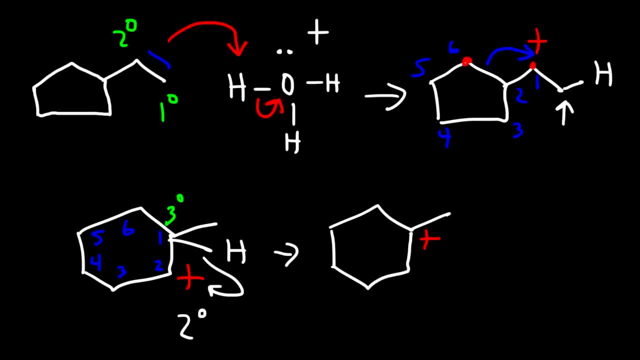 strain. Now for the second part. the hydride shift occurred due to stability as well. A tertiary carbocation is more stable than a secondary carbocation, And so that's the driving force for the second rearrangement. So now the last thing that we need to do is add water to the carbocation. 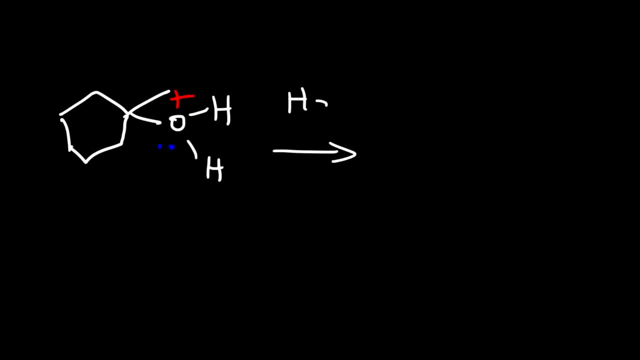 And then, in the final step, we need to use another water molecule to take away a hydrogen, And so anytime you add water to an alkene, you're going to get an alcohol. Now, are there any stereoisomers that we need to worry about in this product? 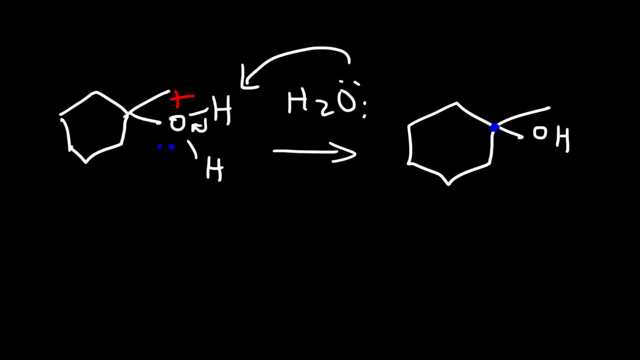 So do we have a chiral center? The left side is the same as the right side, so we don't have a chiral center. Therefore, this is the only major product that we have Now. there could be other minor products, but I'm just going to focus on the major. 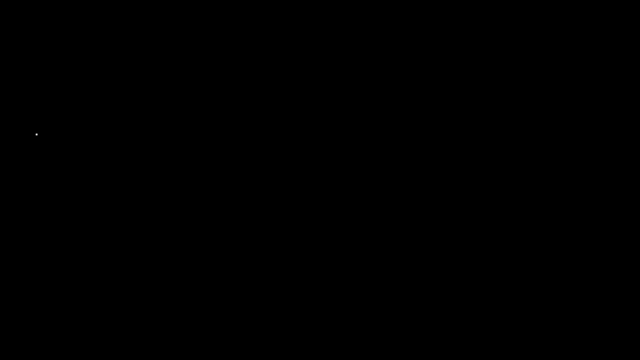 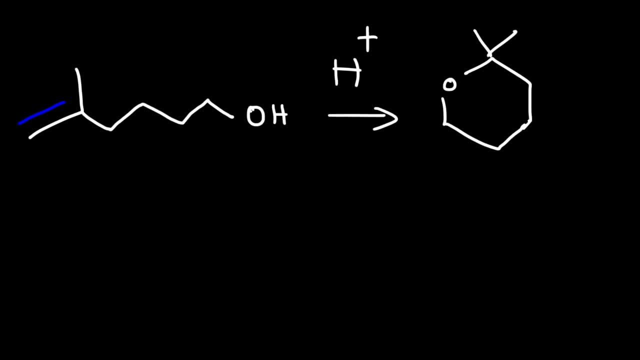 So fill this in, So fill this in, So feel free to pause the video and work on this problem. So what do you think is going to happen here? In order to get this molecule, we need to react the alkene with the H plus ion. 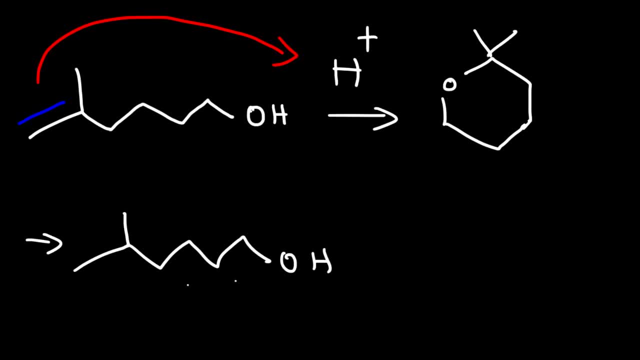 And so we know the hydrogen is going to go on the less substituted carbon atom of the double bond, and this will give us a tertiary carbocation. Now the oxygen has a partial negative charge, and so it's attracted to this carbocation. 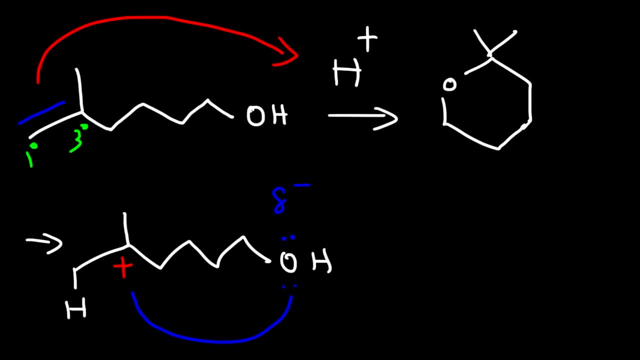 We know that opposite charges attract, so the oxygen is going to attack the carbocation. Whenever you have an intramolecular reaction, such as the one that you see now, the straight-chain molecular structure will convert into a cyclic structure or a ring structure. 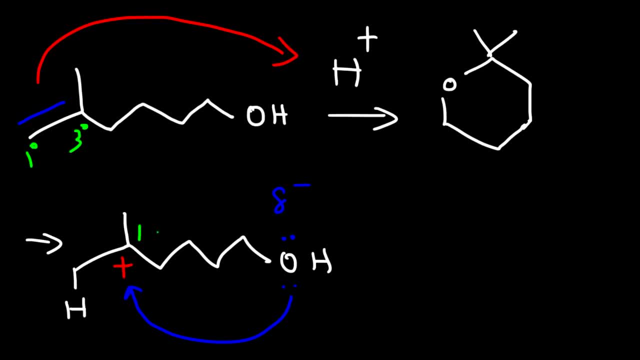 Let's call this number 1 for the ring. Here's the second atom of the ring: number 3,, 4, 5.. We're going to get a 6-membered ring. I'm going to draw the structure that we see here. 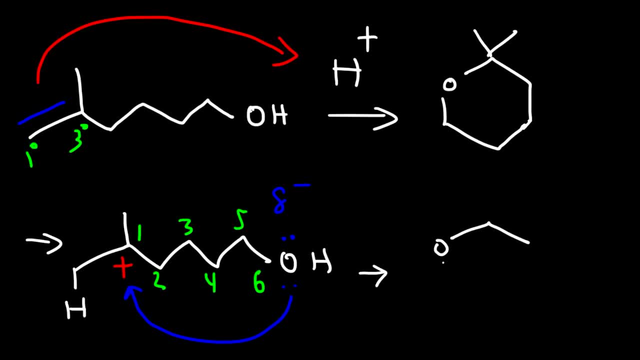 because chances are it's going to look just like that. This is carbon 1.. Carbon 1 is the tertiary carbon and it's attached to the oxygen since the oxygen attacks. This is number 6, which means this is 2,, 3,, 4, and 5.. 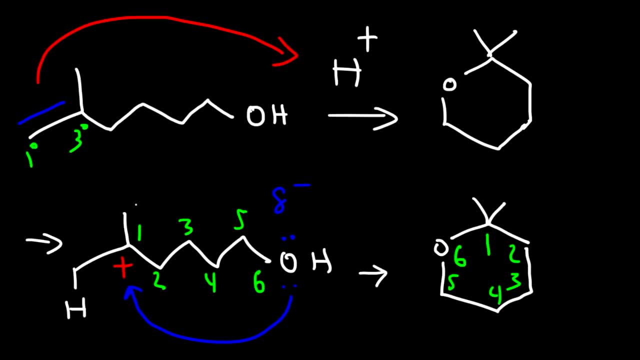 Attached to carbon 1,. we have the two methyl groups, as we can see here. Now what we need to determine is the location of the positive charge. Right now, the oxygen is attached to carbon 5,, carbon 1, and it still has the hydrogen. 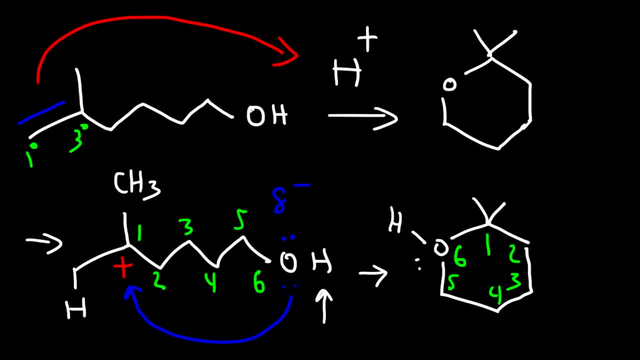 Oxygen has three bonds, which means that it currently has the hydrogen. This is the positive charge. All we need to do at this point is use water or something, some type of base, to get rid of the hydrogen. I really didn't specify. 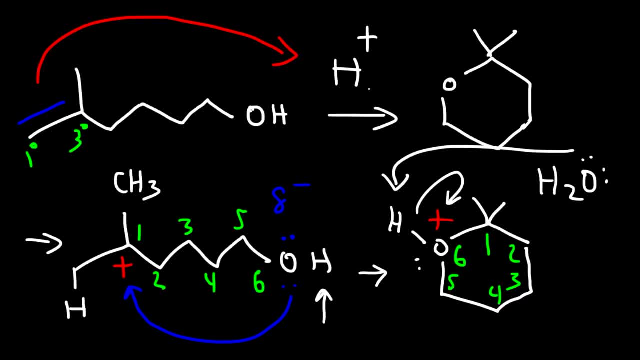 what the solution was made up of. Let's say that it had water to begin with, with some acid. In that case, we can use water as the base On your tests. you might be provided with a different base, So then? 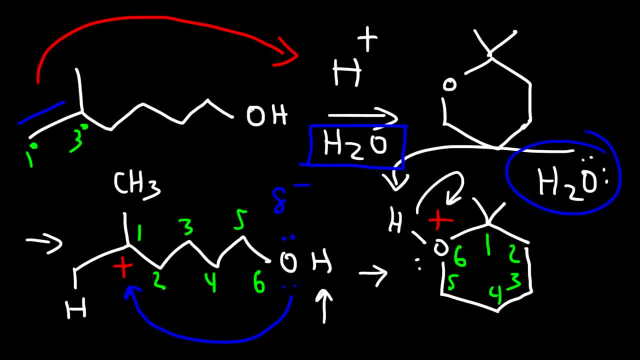 you may have to replace this molecule with whatever the base is Now. granted, we could use the OH group of another molecule like this to take off this hydrogen, So the base that you choose could be many different things. So if we have water in the solution, 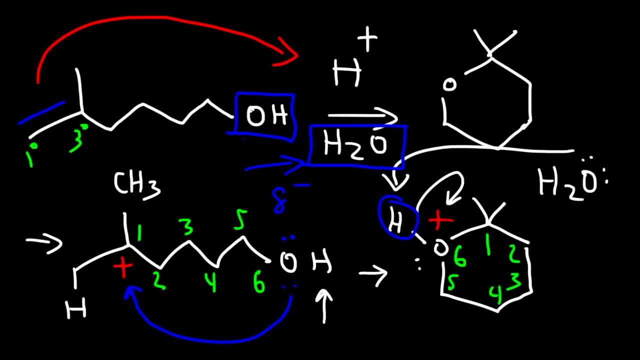 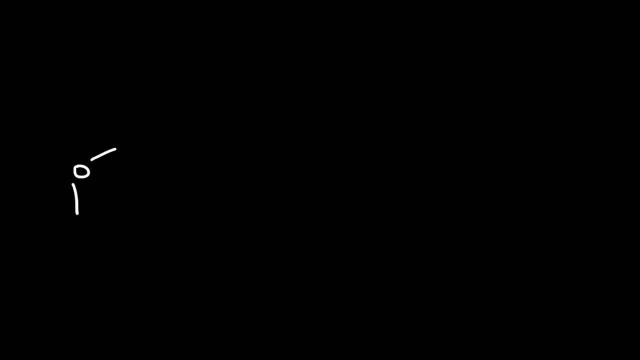 then we can use that as the base. If it's not there, then I would use the OH group to take off the hydrogen. So let me show you. So let's say, if I didn't have water or if it wasn't provided, 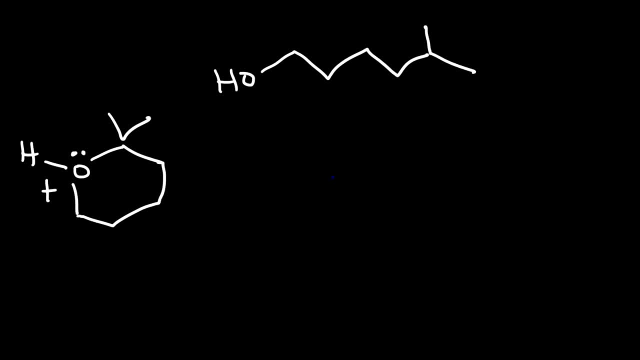 Got to make sure I have the right number of carbon atoms So I can use this alcohol to take off the hydrogen. Either case, I'm going to get the same answer. So there's many different bases that you can use, And so this is my final product.